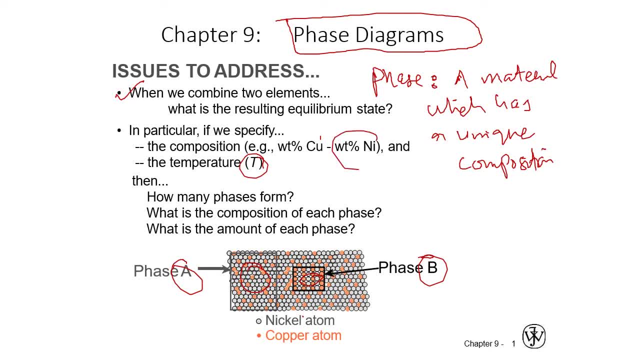 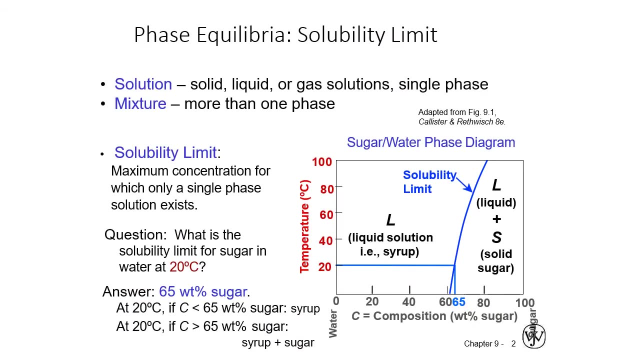 When we are dealing with the temperature and the nickel or the copper percentage weight, Then we can find out that how many phases are there, What are the composition of each phase and what amount of each phase Is present there? So now we can define the phase equilibrium. 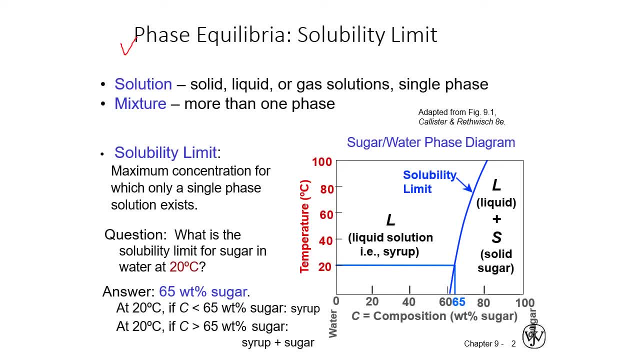 The solubility limit. So these are basically the related terms of the solution. So if I have a solution, For example, I have water And some sugar particles in it, Right, Okay, So the sugar particle is called solute. 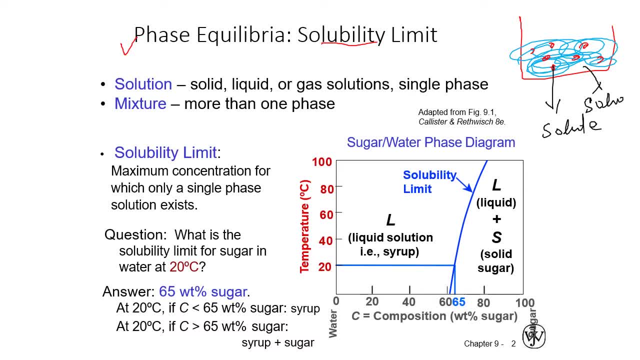 And the water is called solvent, Right? Okay. So solution is basically the homogeneous mixture, Right, Homogeneous mixture, Okay. Homogeneous means that if you take a part from here or from here or from here And you test it in the laboratory, 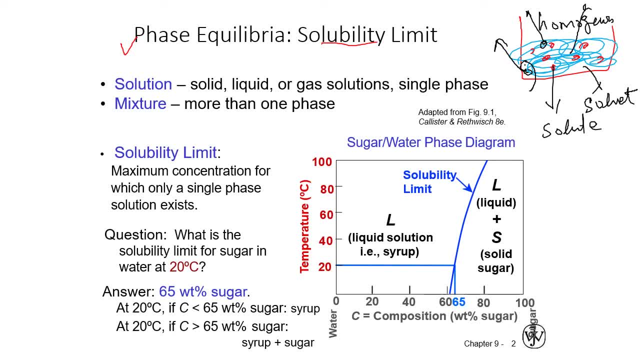 Then you will come to know that It has the same composition throughout the container, Right? So it is called a solution, So a mixture and the solution are two distinct quantities, Right? And a mixture is basically It has, It is basically solution, is its type. 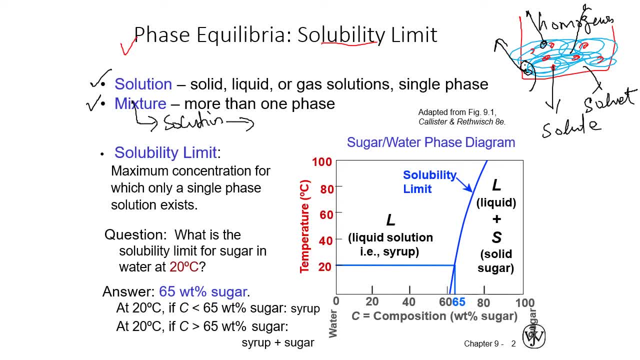 So the homogeneous mixture is called solution And the non-homogeneous mixture Is composed of two or more facets. Right, Okay, So solubility limit. Solubility limit is the maximum concentration of Solute Which can dissolve. 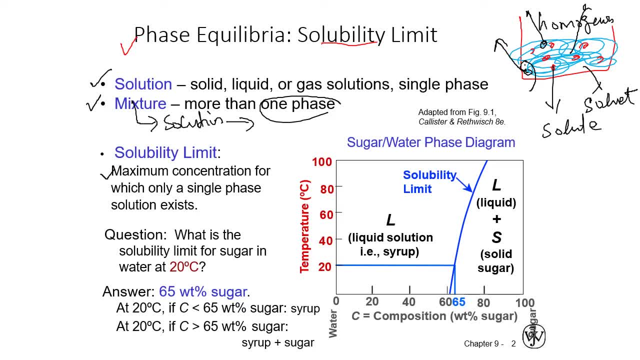 Right. So, for example, where is the solubility limit for a sugar at At a temperature of 20 degrees centigrade Right? So if we look at 20 degrees centigrade Right, Then we see that only 65% of the sugar weight percent can be dissolved in water. 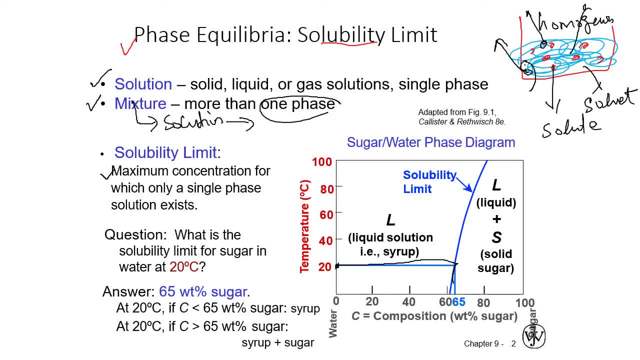 Right. This is a solubility line And we said that This is a solubility limit line, Right. So beyond this, there is only liquid, And if you increase the amount of sugar Right, Then you will see that it will no longer be a solution. 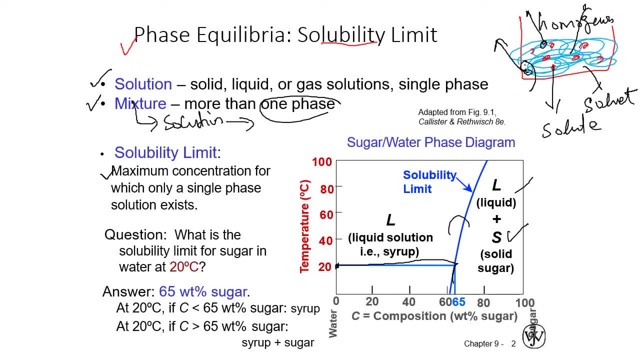 So there are two phases forming Right, And this line is basically separating these two from each other. Okay, So if the sugar concentration is less than 65%, Right, Then it is a solution. But if you increase the, The solution. 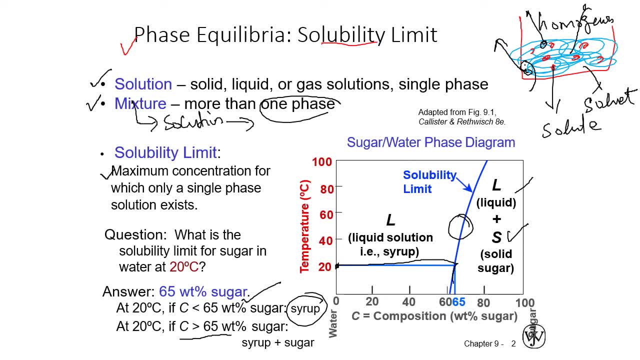 Then it is the syrup plus sugar, Right, Okay, Okay, So what is the difference between the component and the phases? So component is basically the element or compound that are present in the alloy Right And phases. They are chemically distinct. 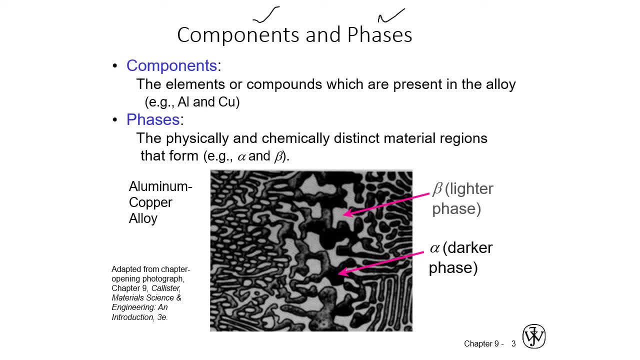 I told you in the previous slide that it is a unique Right. It is a unique Quantity Which has Errors Right. It is a unique Right. It is a unique Quantity Which has Errors Right. It is a unique. 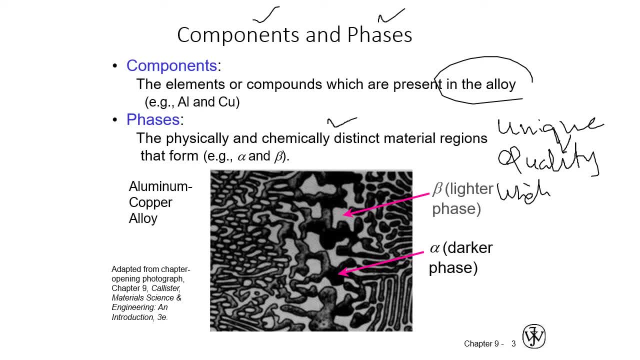 Right, It is a unique Quantity Which has Erm Its Own Composition. For example, When we dissolve the nickel and copper, then we see that there are two types of solids, Right? So one is called alpha solid and the other is beta solid. 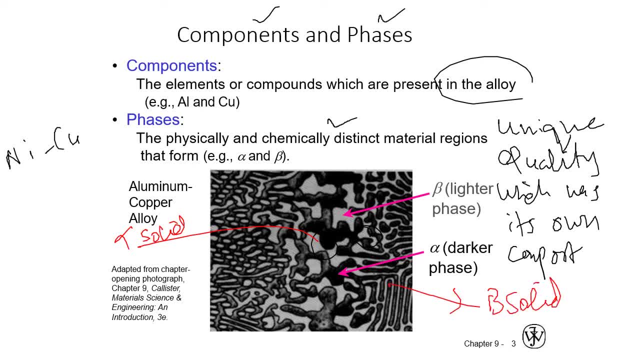 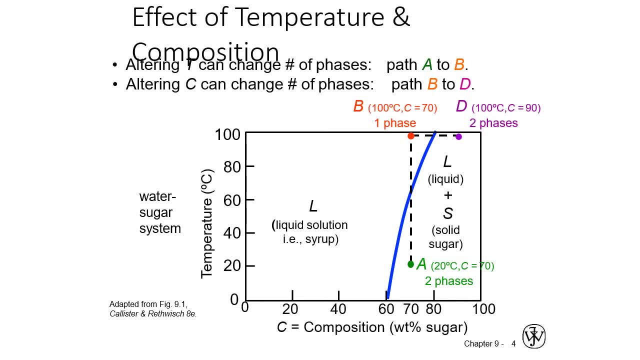 So basically, these alpha and beta are basically the different phases of the same solution, Right, Okay? So now what? They picked up temperature On the composition. So I will show. okay, so if we, if we, if we decrease the temperature from point B to point A and 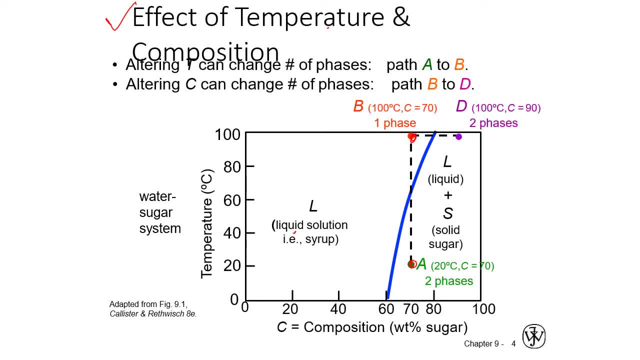 basically, this is again the sugar water solution and the sugar composition is plotted on the x-axis and the temperature is plotted on the y-axis. right, and this is my coordinate system. sorry, it's yx. okay, so this is basically yx and here's the liquid plus sugar. 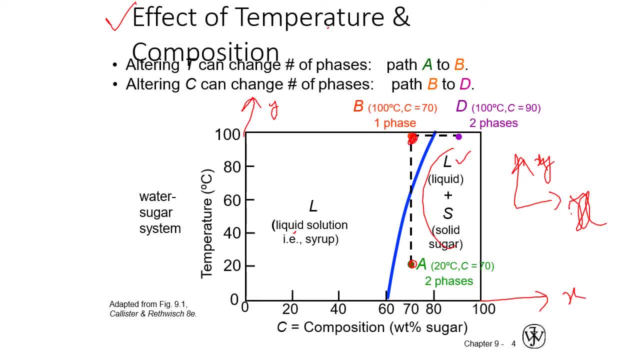 right, and this is the solubility line. so if we move from point B to point a- right, basically we are decreasing the temperature- then we see that we are basically moving from liquid solution to a different phase solution. right, we are entering from syrup to a two phase liquid plus sugar. 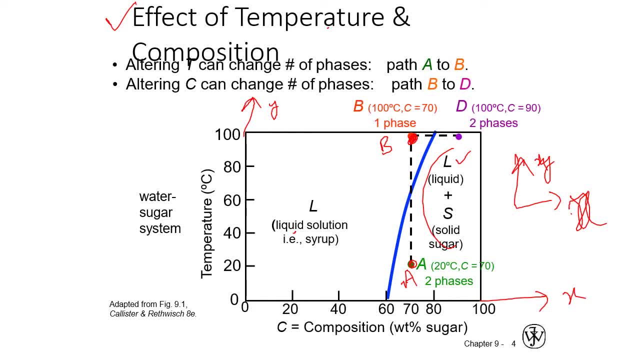 solid sugar solution. similarly, if we increase the composition, we the temperature is remain constant, but if we increase the composition of sugar from beyond the point B, then we see that we are also entering to the liquid plus sugar solution. okay, so we see that the temperature and as well as the 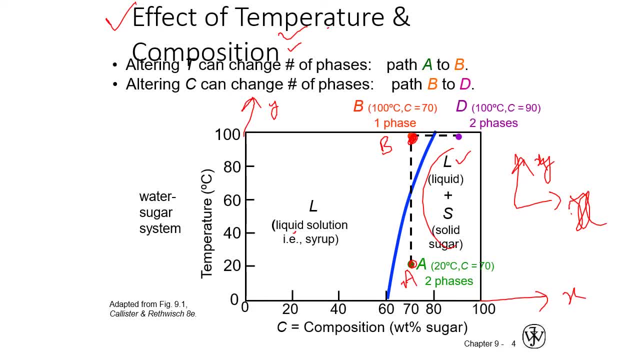 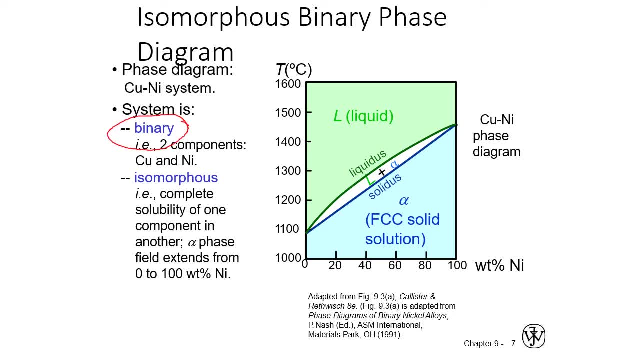 composition effect which passes are present. okay, so in this course, basically you will consider the binary. binary means two phases, right, so at most two elements, two elements will dissolve in each other for the binary alloy. and basically, if you plot the temperature in the composition on the x, 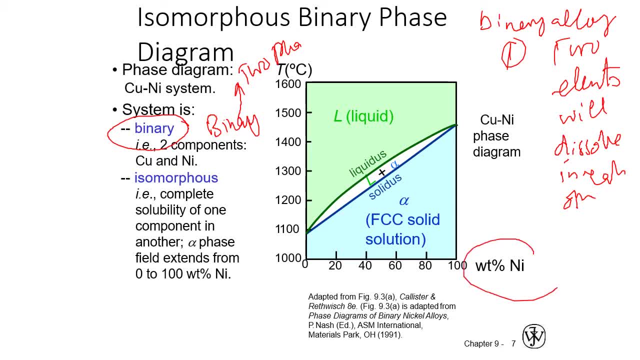 axis for one element and this is called a limiting element, right? so this is an example for the copper and nickel alloy, right? so at specific temperature above which there is a liquid and a specific temperature below is solid and at some point here is liquid plus solid, right? so alpha is basically a solid which has FCC structure, right? and let me 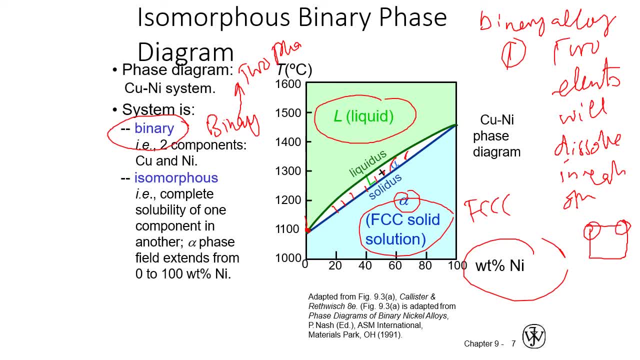 remind you that FCC. look like this: right, it is one element in the face right, and we see that it is isomorphous. right, so will you will see that the nickel and the copper are completely dissolved. right, so alpha phase extend from zero to 100%. we get nickel, right. 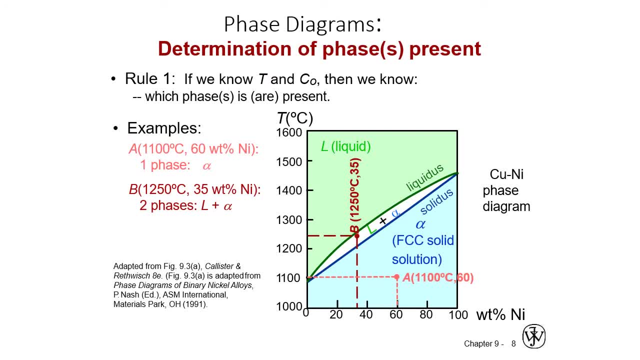 okay, now phase diagrams. phase diagrams basically told us that at which temperature and which composition which element are present. for example, if you are given with the temperature of 11,000 degree centigrade- sorry, 1100 degree centigrade- and 60% weight nickel, then you will see that on the x-axis and 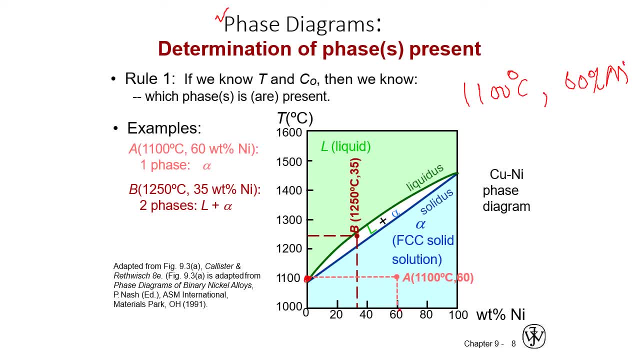 the y-axis there is 1100 and on the x-axis is 1600. so if you meet this point, if you look at this point on the graph, then you will see that it lies in the alpha solid region. so you can say that at this instant. here is 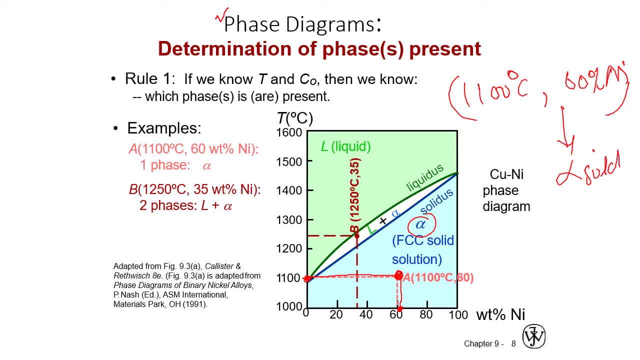 also the alpha solid region. so you can say that at this instant here is also the alpha solid right and if you are given with the 1250 degree centigrade temperature right, temperature is 1250 degree centigrade and the nickel weight composition is 35% and you locate this point right, so you will notice that it. 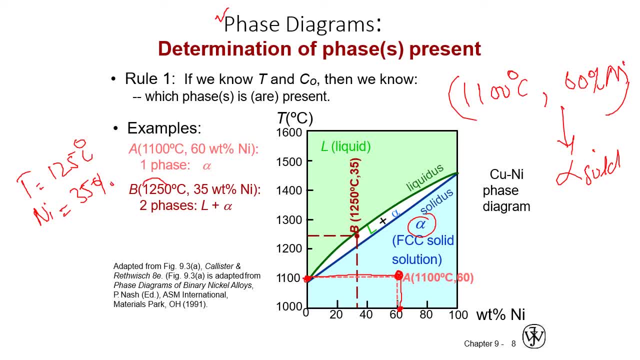 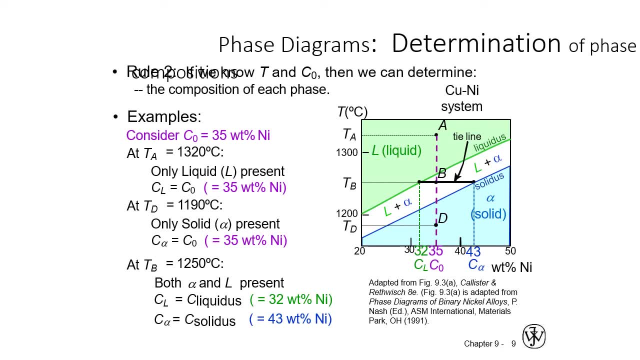 lies in the L, the liquid plus solid region. okay, okay, now we are given with the liquid plus solid region, and now we are given with the problem that we should- you should- determine the phase when you are given with the temperature in the composition, right? so in the first, 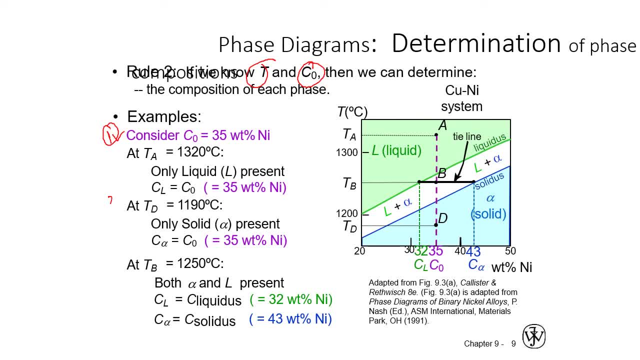 example, this is first and second, this is third right. so you are given with the weight percent of nickel, which is 35%, and at 1320 degree centigrade right. so basically this is 1320 degree centigrade right and this is 35%. so if you join the vertical and horizontal, 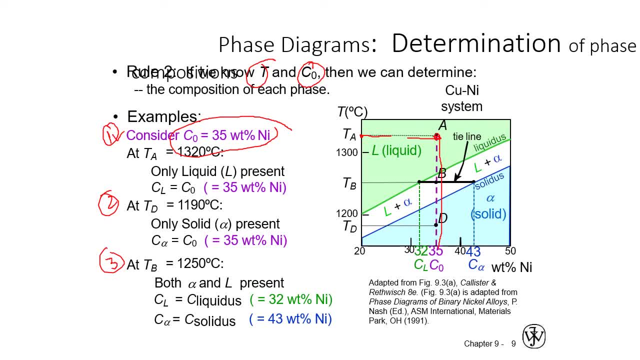 line, then you will end up at this liquid phase, right, and if you move down with the temperature of 1190 degree centigrade, right. so this is basically a constant composition line and if you move down to this point, then you will see that there are two phases basically present, right at 1250 degree centigrade and at 1190 degree centigrade. 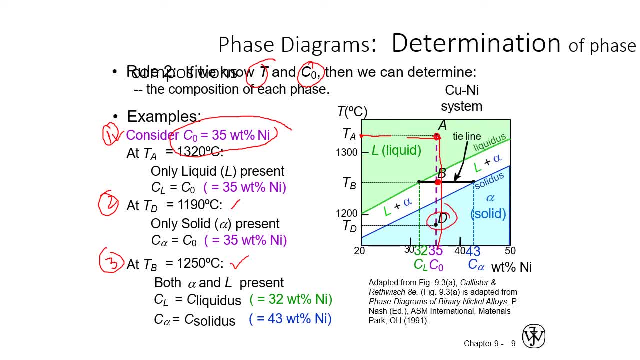 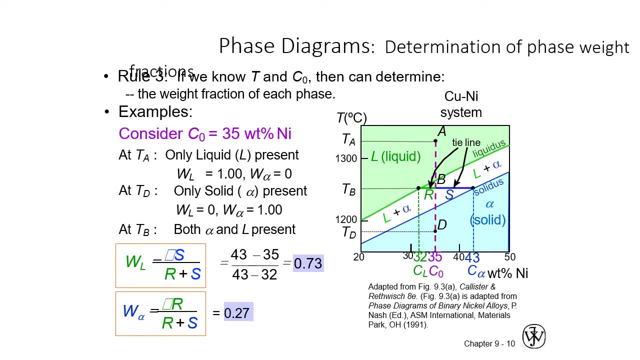 degree centigrade, you will see that only the alpha solid is present in this solution, okay, okay, so the phase diagram. we can determine the weight of each phase, right, okay, so if you are again with the temperature and composition, you, then you can determine the weight person composition: okay. so, for example, if you 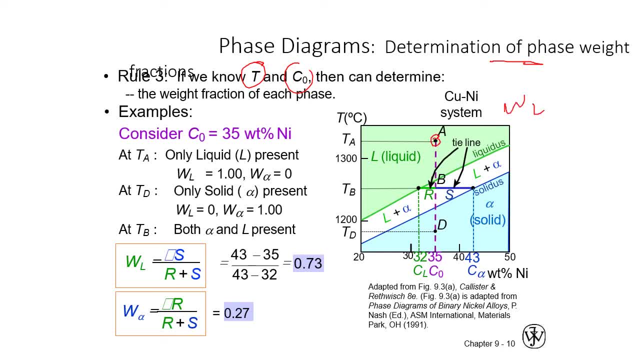 end up with the point A, then you will see that the weight percent of the liquid is 100% right because there is only one phase. and at point D the weight percent of the alpha is also hundred percent and the weight percent of the liquid at that point is zero. similarly, the weight percent of alpha at 1100, at 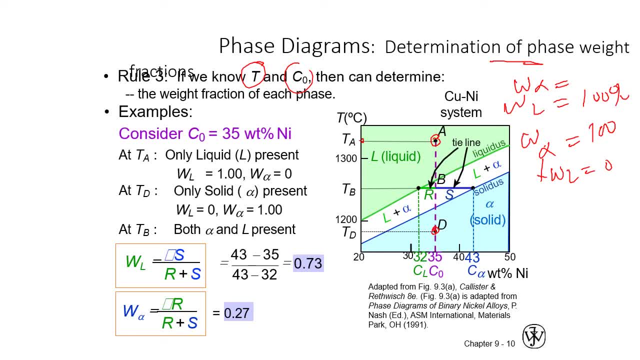 sorry at at this point. right, this is 1320, it is zero because there is no solid and there is no liquid at g point. but at b point we have an interesting phenomena: we have the liquid plus the solid. so how can, how can you determine these? well, for this. 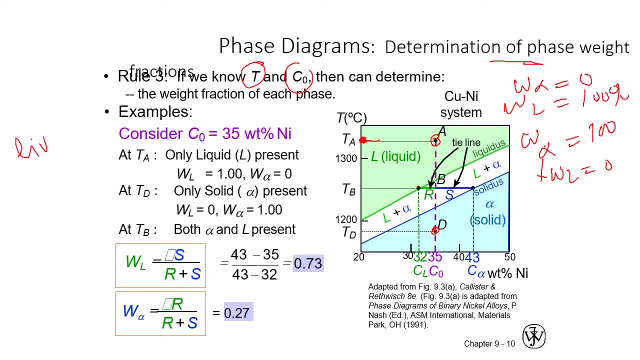 basically, we use the lever rule. right, lever rule, lever rule. okay, so if i, if i zoom out this section to here, right, then you will see that this is the liquidus line, liquidus line, liquidus line means that above this, liquid will start, right above this there will be liquid, and this is the solidus line. 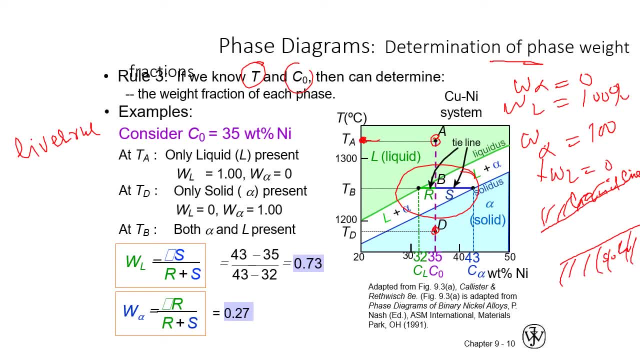 so you will see that below this all the composition will be solid right and in between there will be l plus alpha right. so, for example, if you end up at a point b, so this is my point b right, so you will draw a tie line. tie line you will extend from one, from point b up to the liquidus line. 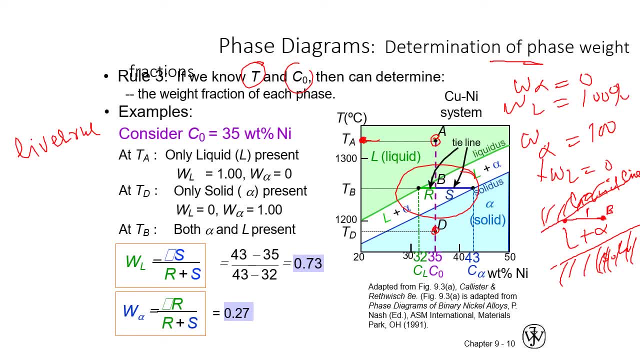 and you will call this distance as r right. and you will also extend this line to the alpha line right, and you will call this distance s right. so now, if you want to determine the composition of the solid right, so for the solid you will write at r w of alpha equal r divided by r plus s right, and for the liquid, you: 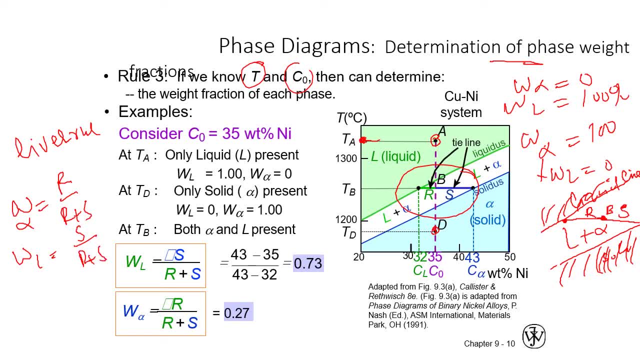 will write s by r plus s, right? okay, so now determine what is r and what is s. r is basically the distance from point b up to the liquidus line and, under composition, x-axis distance. so you will see that the r addition is basically here 35 minus 32. 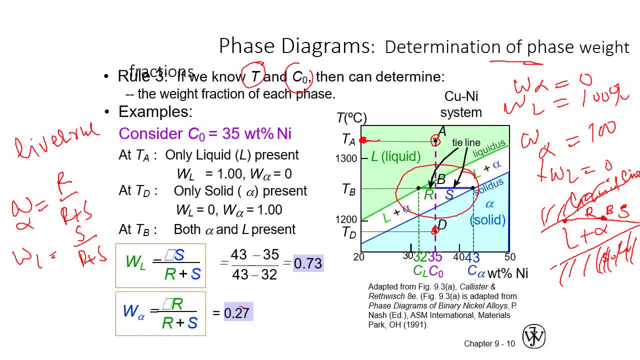 right, 35 minus 32, so it is basically 3, r is r is 35 minus 32. divide by. and what is r plus s? this is r and this is s. so r plus s is 3 and r is 32. so we can calculate this. zero çıktı Instagram. minus thirty negative pu by. and what is r plus s? this is r and this is s. so r plus s is negative. pi division is 34, communities33. Hypothetically, R-32 Is the point, brn is 1, Lucy Min and two million areas are negative. So you can get as interval for every dimas and chemistry. in the application for the next lesson we will check for this example. 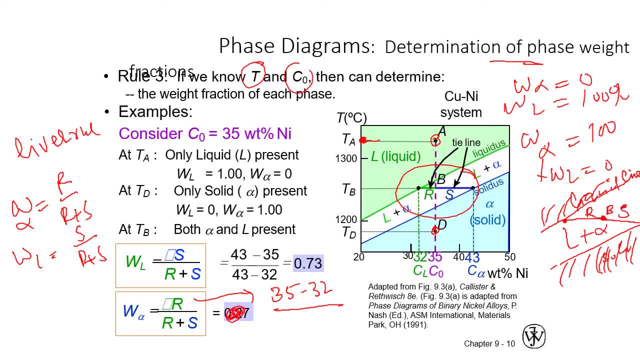 is 43, right, and minus 32, 43 minus 32. so if you propound this calculation, then it will come out to be 27 percent, right? okay? so since here are only two solids, right, two phases, so you can determine the composition of the solid. 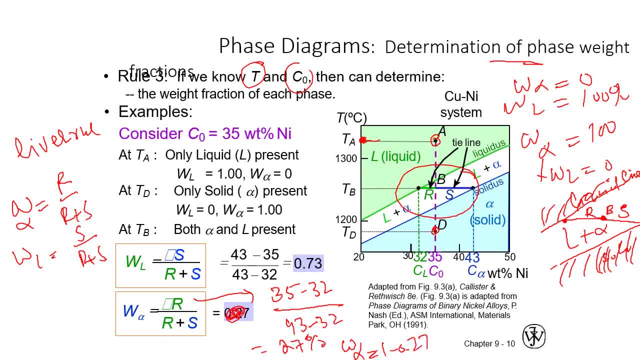 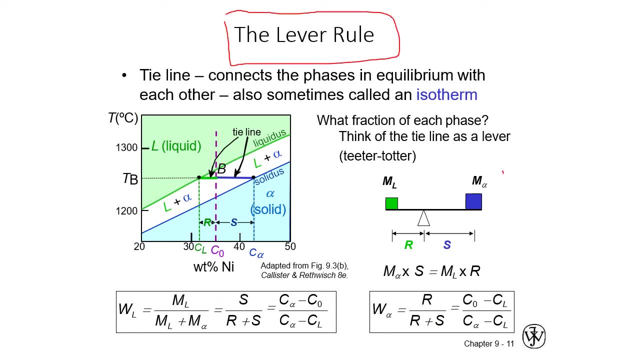 as W alpha equal 1 minus 0.27, which will be 0.73, right? or you can say it is 73 percent, right, okay? so on this slide I have explained the lever rule, right? so what is our lever rule? basically, this is this is explaining that: how can we determine the composition of the solid? 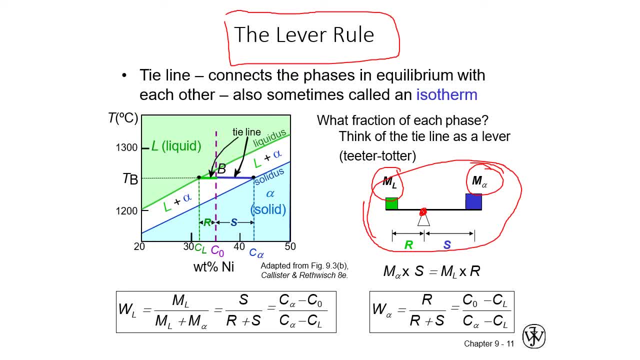 and the liquid right. so you will see that this is the pivot point here- both the liquid and solid are balancing each other. so this is basically the R distance and it is the S distance. so if you take the moment about L equal to 0, then you will. 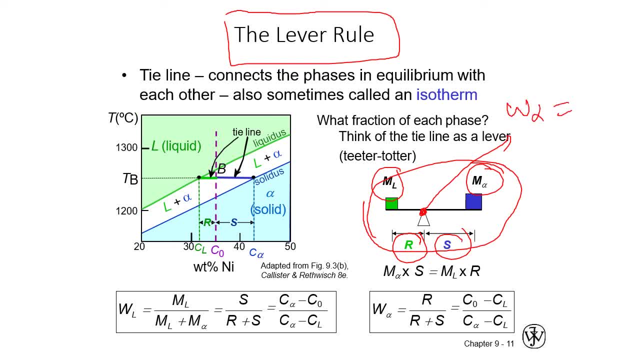 notice that W of alpha equal R divided by R plus S right. and if you take the moment about about this point about alpha equals 0, then you will notice that W of L equal S by R plus S right. so this is basically the lever rule. that how can. but the trick point is here is that that you will come. 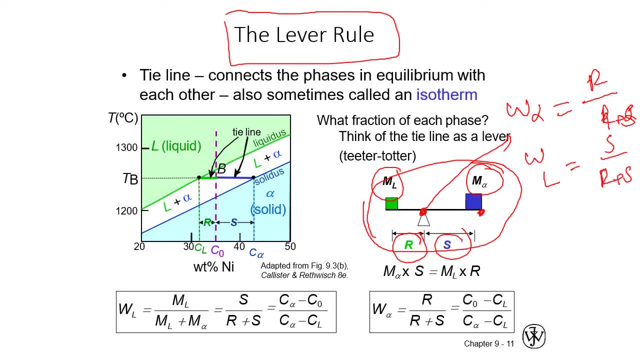 you will consider the opposite direction right. for example, if you are, if you want to determine the composition of the liquid, then you will consider this distance divided by this total distance, right. and if you want, if you want to determine the composition of the solid, then you will divide this distance. this distance is here R and the whole. 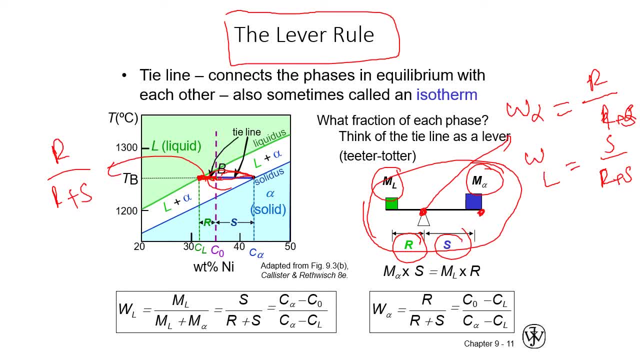 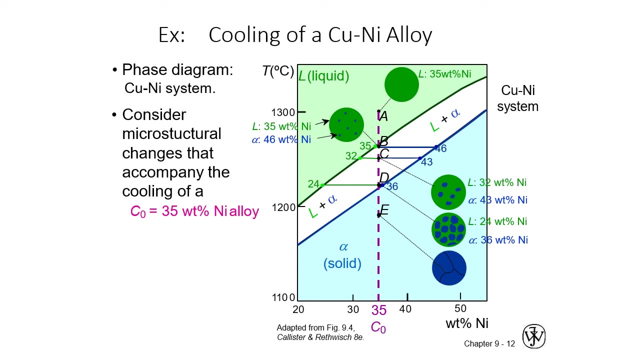 distance is R plus S, right? and similarly, if you want to determine the liquid concentration, then you will divide the S divided by the total distance, right? so this is a trick. here. it is basically opposite and the composition has been explained here, right? okay, so on this slide, if you cool down this copper and nickel alloy along the 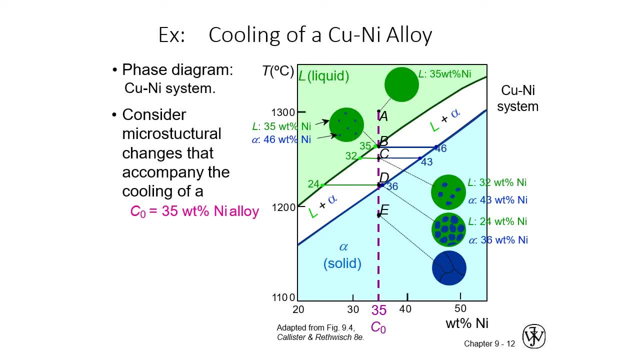 constant composition with respect to temperature, then you will notice that the liquid and the solid, how the solid is forming okay. so if I am at point A, right at point A, if we move out some portion of this alloy and you notice, you observe in the microscope, then you will see that all the composition is liquid. 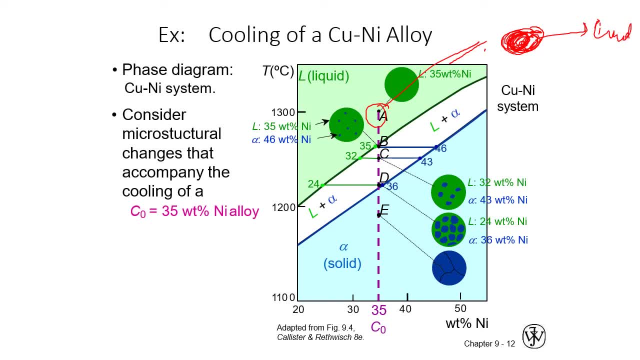 right, so this is liquid. okay, so when you, when you reach this liquid is line, right so you will notice that these microstructures are forming. so this is basically the start of formation of the alpha solids. and when you go beyond the liquid is line at point C, then you will notice. 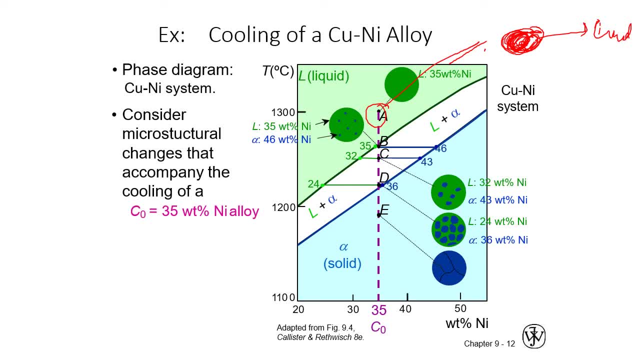 that these small particles of alpha solid, they are basically increasing right, they are basically increasing in size. and also you will notice that the composition of nickel is also decreasing right in the alpha solid and it is also decreasing in the liquid right. but if you move to the point D then you 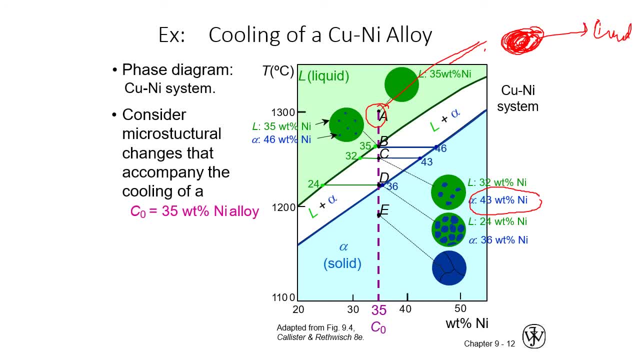 will notice that all, almost all of the liquid becomes the solid. and when you reaches to point E, then you will notice that it is all solid. power alpha, right, power alpha. okay. so it has the composition of nickel. nickel is 35% here and the copper is. copper is 1 minus 35, right? 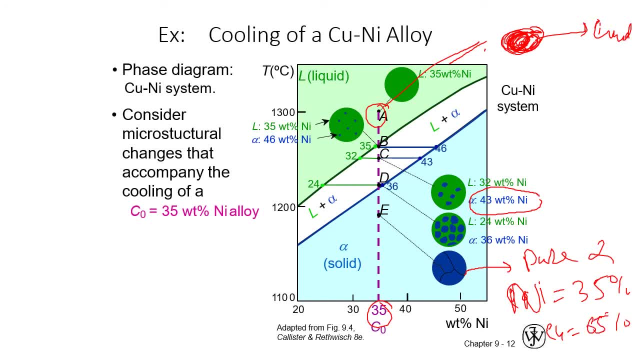 100 minus 35, so copper will be 65%, right? so this is the final composition of the alpha. so you notice that how, with respect to temperature, the composition of the alloy changes, right? so they're basically a point for us that if we control this cooling, this cooling, then we can form the structure which has a 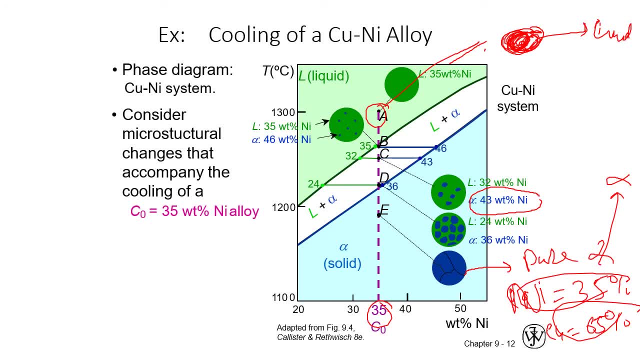 specific strength and which will affect its mechanical properties also. okay, so that's it for today. see you in the next lecture. thank you.